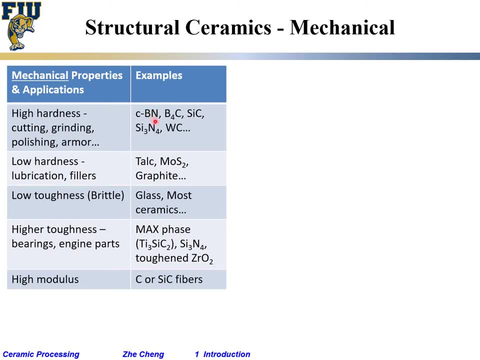 cbm for so-called cubic boron nitride. repeat with me quietly yourself: cubic boron nitride. okay, it's boron and nitrogen, or b4c boron carbide, or silicon carbide or silicon nitride or tungsten carbide. the list go on and on and on. but for 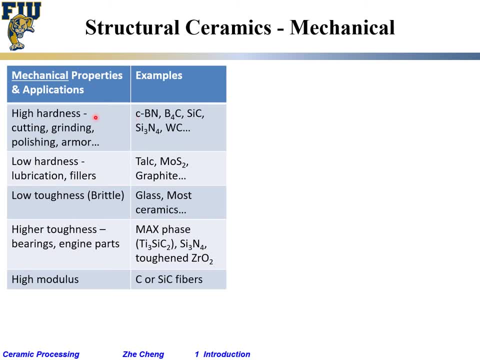 all these materials, quite often we utilize the one mechanical property, a property probably more, but i'm emphasizing one so-called high harness. okay, i'm showing one example, a picture of an example. what is this? it's a bag of a soldier or dummy soldier, and this piece can be a so-called armor- bulletproof vest or helmet, bulletproof helmet and quite. 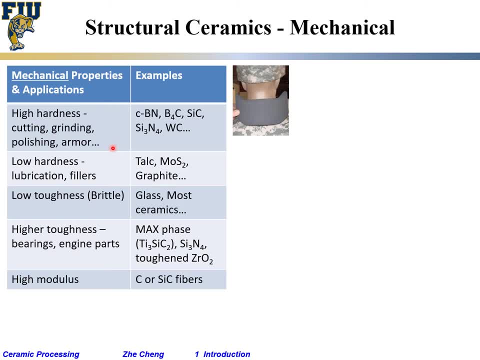 often nowadays, the armor is a composite, but in the so-called striking phase, the phase that is going to face the bullet first, will be ceramics. why? because it is very, very hard. okay, and i'm showing the second one: mechanical engineer. what are these? the cutting tools put it, you put it on a machine and when it rotates, 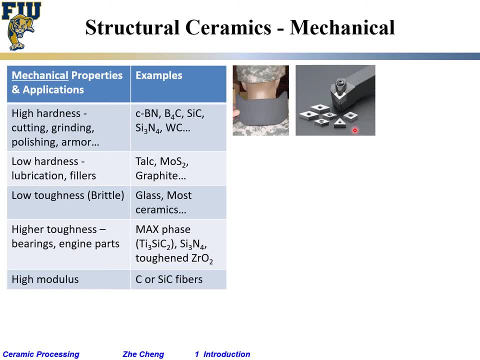 okay, and i'm showing the second one: mechanical engineer. what are these? the cutting tools put it, you put it on a machine and when it rotates, these types of bits cut into whatever material: could be copper, could be steel, could be hardened steel, martensite hardened steel, very, very hard steel. how do you cut them? you're going to use something. 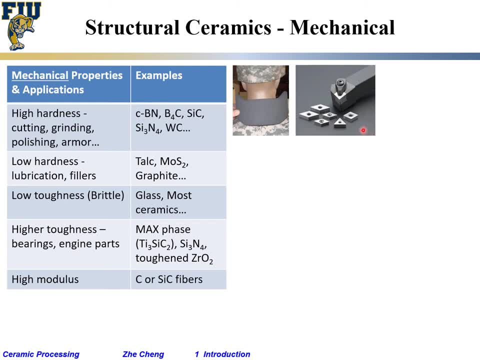 harder than those hardened steel and those harder material could be diamond. but sometimes diamond doesn't work. people have to use some other material like silicon nitride, tungsten carbide or cubic boron nitride, very, very hard material. hard is only next to diamond and people make them into these. 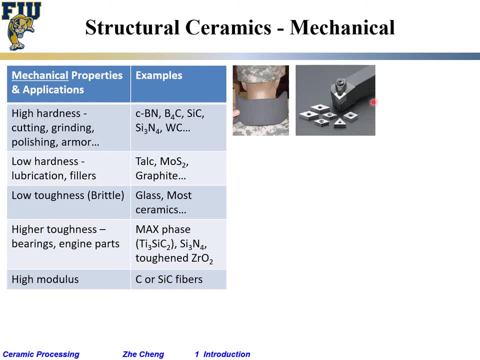 shapes mounted onto your tool and use them to fast machine cast iron or many other material hardened steel which are very, very hard, makes sense. so these, you say: okay, i can machine copper, aluminum with steel. to machine steel, i can use so called tool steel. and then what material am i going to shape my tool steel hardened to steel? well, you have to. 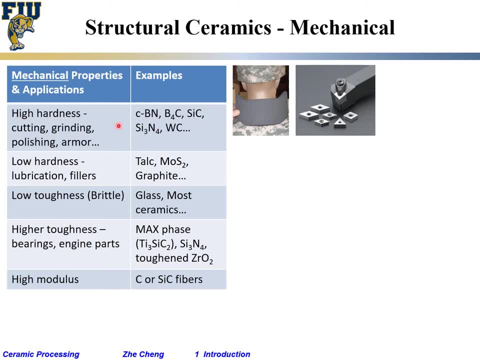 use something harder, which diamond or something like these types of ceramics make sense and the reason people move initially from like nitride to carbide and then to cubic boron nitride. the harder your material, your tool can last longer or shorter, the harder your material tool can last longer and 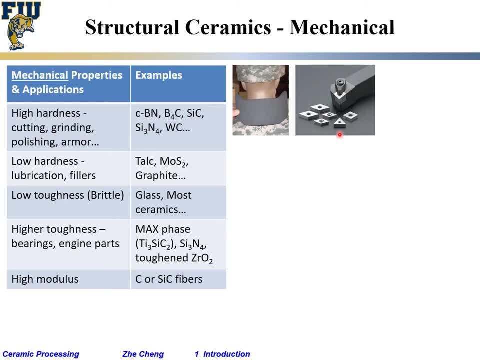 quite often you're machining speed can go far faster or slower. faster you are machining speed can go faster your productivity goes. which way higher, right, if you're gonna machine cast iron, if your tool is soft, you can only go so fast make sense. productivity depends heavily on hard material. 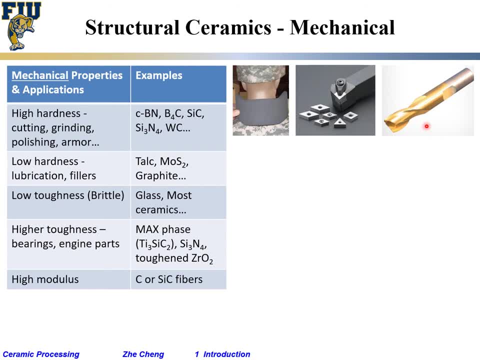 okay. and then i'm showing you what mechanical engineer drill bit right quite often drill bit. most of the time the machine goes faster or slower and this material depends on the material. and then i'm showing what mechanical engineer drill bit right quite often drill bit most of the time. 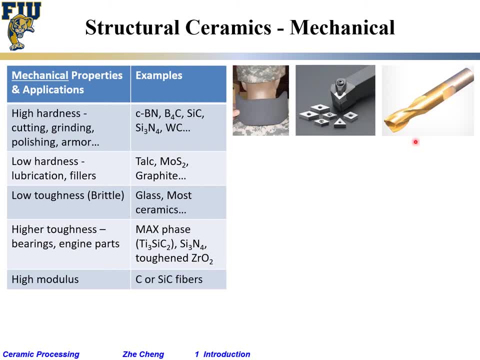 most cases, the drill bit, the inside, is a hardened steel, but quite often, to make it even more well resistant, you sometimes find this gold color. what is that gold color? any metal is goldish. well, you said gold is goldish, but are you going to apply gold onto a drill bit? 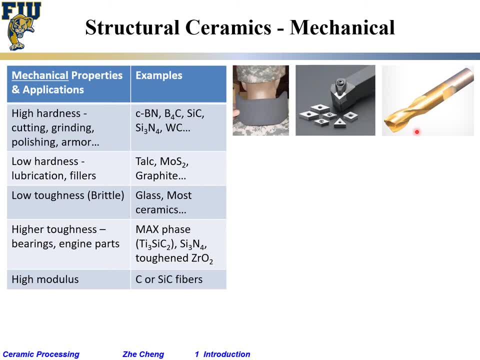 or copper on your drill bit? no, why doesn't have? it's too soft. so what essentially people put on here? this goldish color is actually coming from a ceramic called titanium nitride or some other types of coating material. ceramic, all ceramic. why to make the drill bit the? 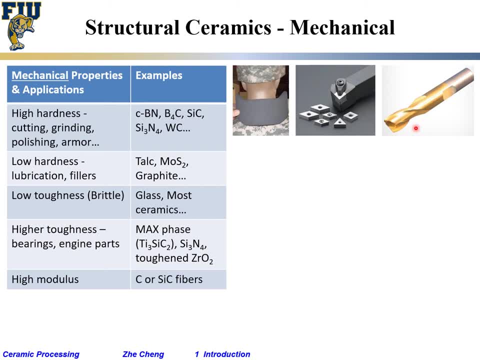 harness maintained so that it lasts longer, i can drill faster, make sense. and then i'm showing all these. what are all these for mechanical engineer? these are sanding wheel, sanding paper, all of them. and quite often the paper is not the one that does the job. it is what it's: an embedded particles. 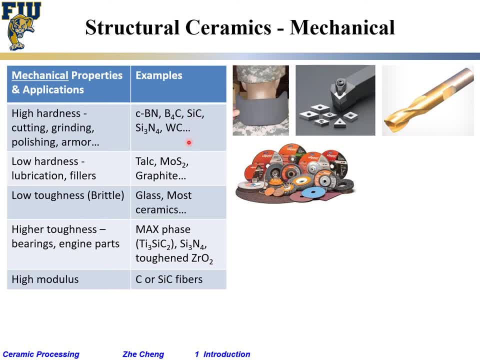 which are often silicon carbide, could also be tungsten carbide, embedded well into the wheel, into the paper, into the pad or diamond that does the cutting, grinding, so that you can make the material, what typically metal part, what smoother right, reach certain roughness you specify for certain friction or whatever application make sense. so all these materials, 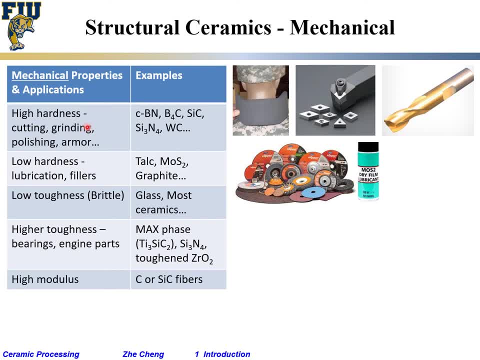 we are using the property of high harness but, on the other hand, for some other cases, we are using ceramics for their read to yourself. low harness for lubrications, for fillers. okay, the materials that are listed here are graphite hard or soft graphite- soft. right, you can use graphite and 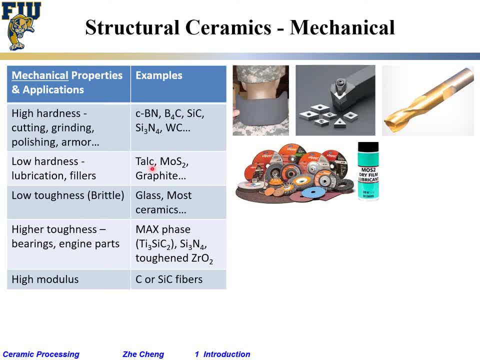 lubricant, believe it or not. you can also use some other material, like torque, soft or moly sulfide, moly disulfide, which i am showing one thing here. you saw this product. it says mos2, moly disulfide. what dry film lubricant, which means the material. this moly dies sulfide is hard or soft. 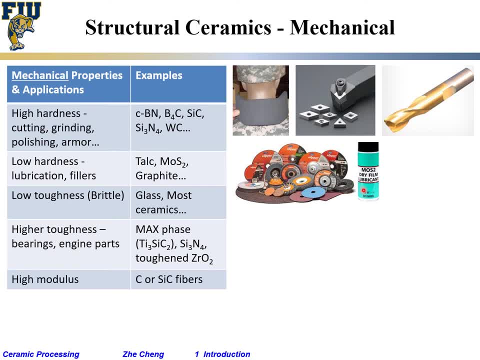 soft, lubricant it when you add it there, it helps the material to slip past one another. so you see, some ceramics are very hard, some ceramics are very soft, very, very soft, very, very soft. okay, okay, let me okay what i'm showing here, these two. i'm showing a types of so-called ferrule. 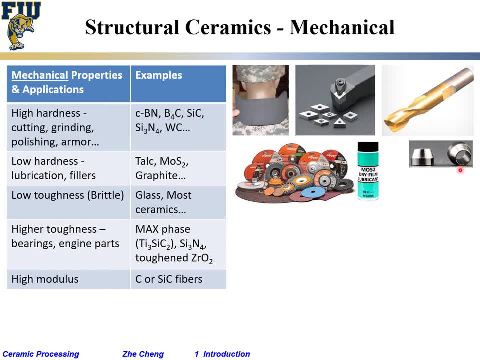 what types of material if you have. you have to guess what i have to guess: black graphite, graph, item ferrule, and graphite is hard or soft, soft and people put graphiteamy, zoals maka it, around a glass tube, earned glass tube or a ceramic tube, and then, when you tighten the 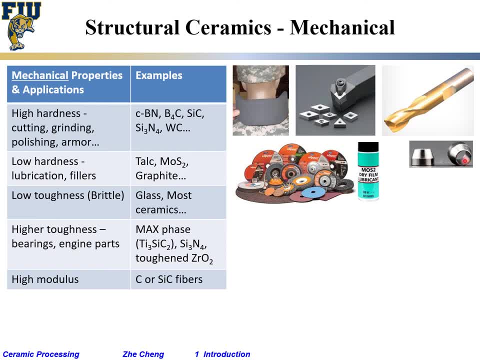 graphite would form the seal- common Styrofoam seal- because graphite is very soft and self-lubricating. when you tighten, the graphite will form the seal. so because grab it is very soft and self lubricating, when you tighten the graphite is very soft and self lubricating. 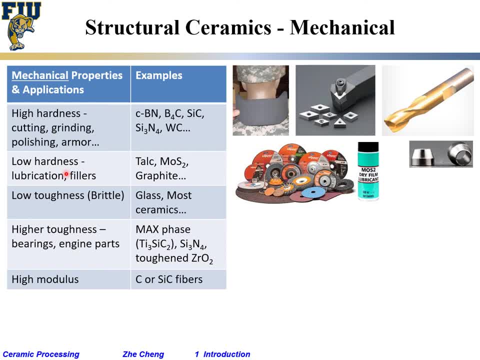 tighten it it can seal onto a brittle material. make sense if i have pass a glass tube through this hole. if i use a metal ferrule, when i tighten that metal can easily what crack the glass tube. but if i seal the glass tube with the graphite- or sometimes polymer but graphite- 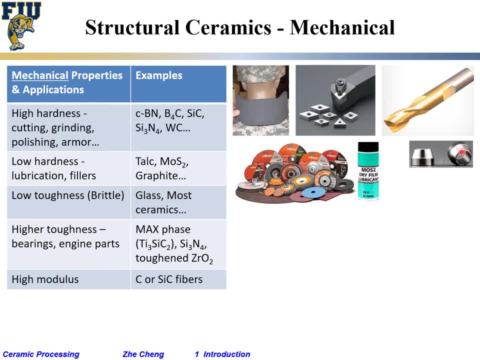 can handle higher temperature than polymer make sense. so if i want some seal at 450 degrees c 500, i can only use graphite. i can use graphite. make sense to form the seal around a brittle material. make sense. so these materials we are using, the so-called low hardness okay. 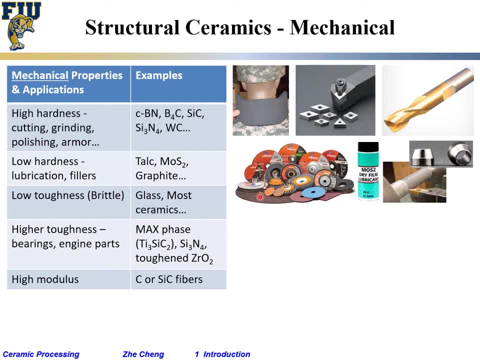 and then some material, ceramic material, most of them. we know most ceramics are brittle, low toughness, right, most of these, these are coatings or this one, if you hammer it it's going to crack, but some of them ceramics. they have higher. i would only say not high, but higher, higher. 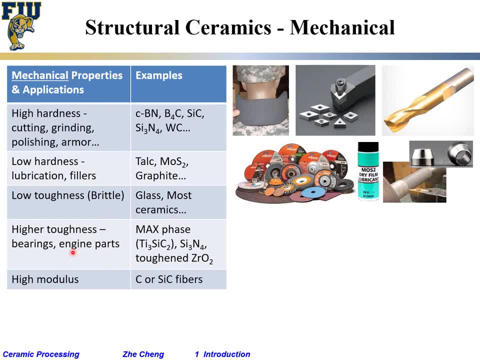 than typical ceramic, higher toughness. they can be used for bearings engine part. here i'm showing a ceramic called the max phase titanium silicon carbide- ti3 312- titanium silicon carbide. this material people can put in a glass tube like this. you can see that it's very hard to put in a glass tube. 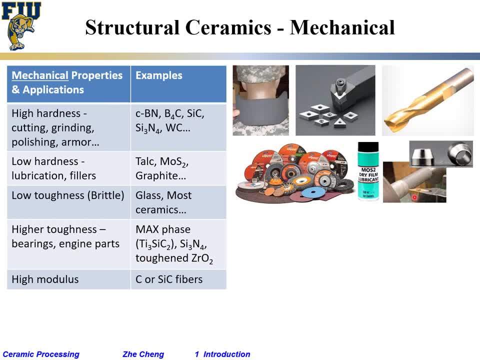 you can put them onto a machine lace, for example, and put your tool ceramic to harder ceramic and start to machine it pretty fast. typical ceramics: you cannot do it easily because it tends to crack, but this material, titanium silicon carbide, can have decent toughness that allows you to do machining make sense. 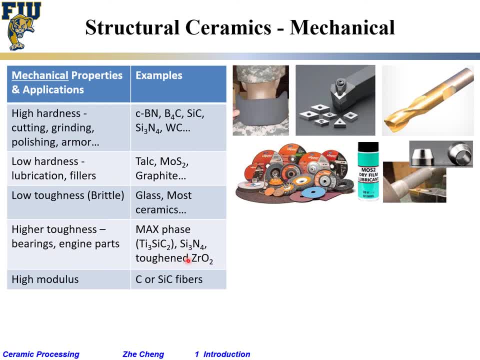 or some other material, silicon nitride or toughened zirconia. what i'm showing here are for mechanical engineer bearings, ball bearing- all types. but when you look at his, what is this material that? typically it is not a. as you look at it, does it look like metal? at least these. 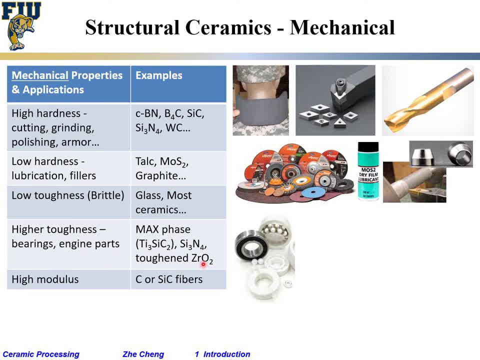 no right, these are zirconia, toughened zirconia ball bearings, ceramic ball bearing, and there are other bearing made of silicon nitride. believe it or not, there are high-end bearing for special application that allows the bearing to go extremely high. revolution. we are talking about hundreds of thousands per rpm, hundreds of thousands rpm. it's really really. 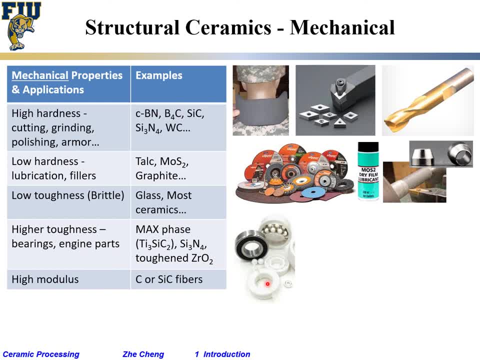 really fast. why? because they don't soften as much as metal. make sense: yeah, we stand higher temperature and the friction coefficient of friction is very, very low. make sense, so for only for special application. you can imagine. these are quite often much more expensive than many typical metal bearings, but you use them for special application. that is very, very demanding. 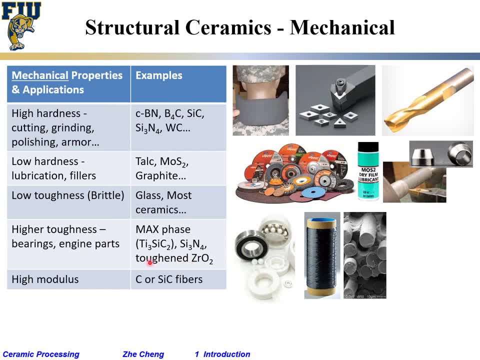 make sense. okay, and for some ceramics, people use them for their high modulus. here i list the carbon or silicon carbide fibers. what are these? these are fibers. you put it around a wand, right? you see that it's like a a, a thread onto a cloth or something. you want that up, and then people. 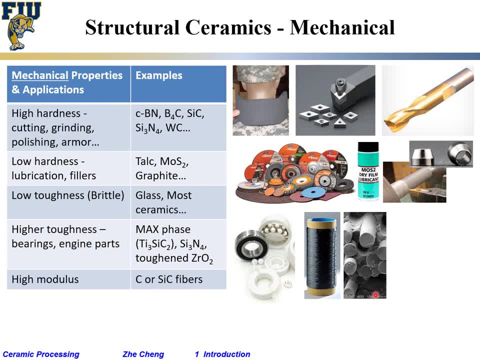 can make this fiber into so-called composite. do you see? this is fiber, but embedded with something else. diamics, competition isLa. but how can we make this component? by using imagem in Na Coun graves of silicon carbide fibers and their proportion of uhanza但是 Yeah이드 of silicon carbide fibers. carbon, Sie traz metal to make the material white hotter than the surface. once a bond silicon in Na provide ahinda of new child cool after theulus that scratch vaseline of a ring of and vibrance. silicon and marking, forgive wind layer, illusion of thickness, cross of hover, iron, or erzählt that this things are very good characteristics. 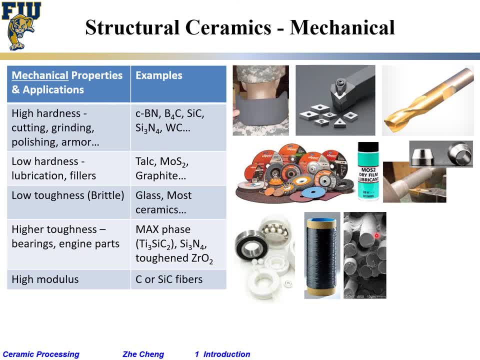 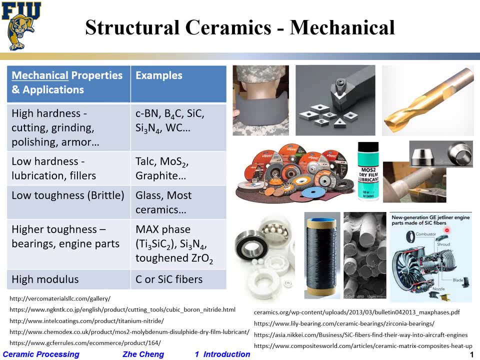 silicon or can be other polymers, make sense. people make them into a composite and well, do people use them? well, people use them, if you see, for jet engine purpose or for some very high-end aerospace properties. that's, i would say, a quandary, but it's very, very. 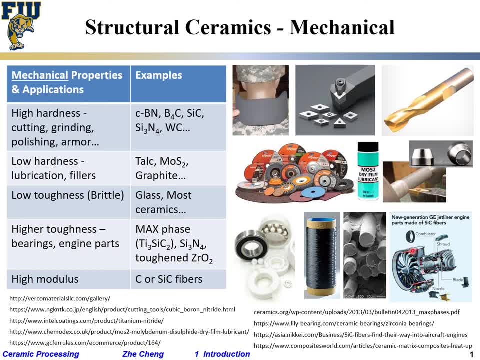 tough, very, very tough right for engine part companies such as GE or some other company. they're trying aggressively for many, many years now. finally they're starting to put some CMC ceramic matrix composite reinforced by ceramic fiber- could be carbon and maybe silicon carbide fiber in there into the engine part. the advantage is very obvious. 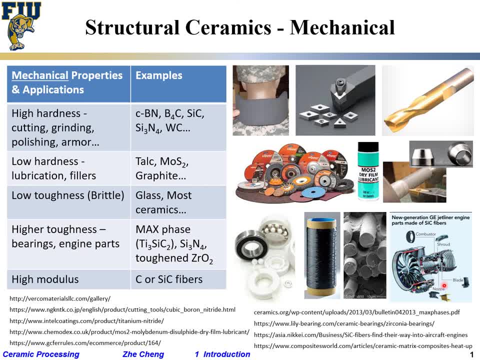 typical engine part made out of so-called super alloy. the density is much, much higher, double, triple of ceramics. the melting point is lower than these types of ceramics. that's the driving force. if you can somehow get the engine not off them, but at least some part of it, replace the metal with. 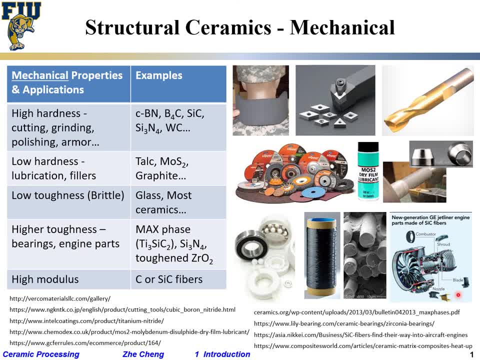 ceramics. the weight goes down, the combustion temperature maybe go up a little bit. for mechanical engineers combustion temperature goes up, weights goes down. that helps my jet engine efficiency right, make my airplane go faster, make sense. so that's kind of a fundamental. a lot of these technical applications quite often are limited by some types of material. 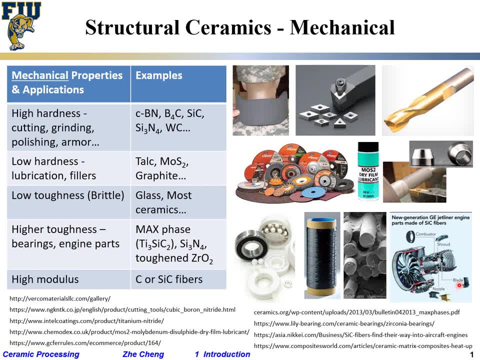 that's why people are investing so heavily into material and, in our case, into technical ceramics. okay, 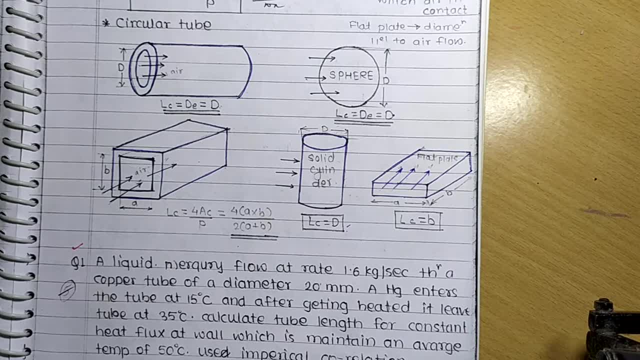 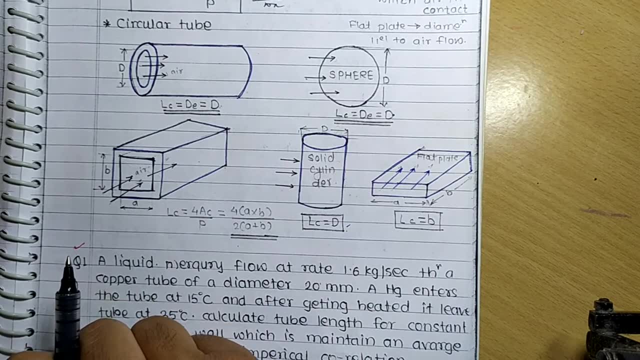 Hello friends, welcome back to my new lecture. Today we are going to solve a problem on a force convection. When we are going for solving a problem on force convection, we must know what is characteristic length, Because in the force convection we are having many dimensionless.